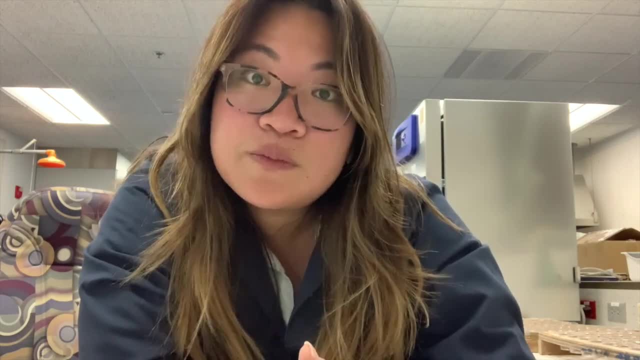 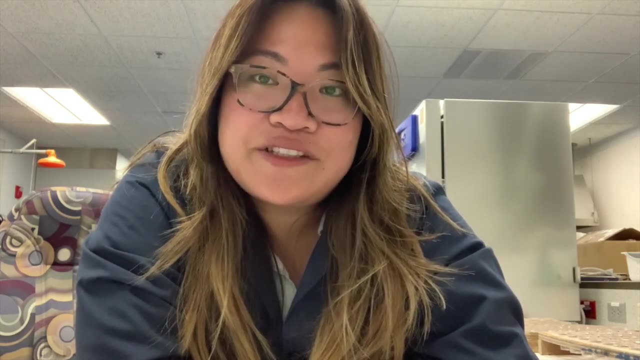 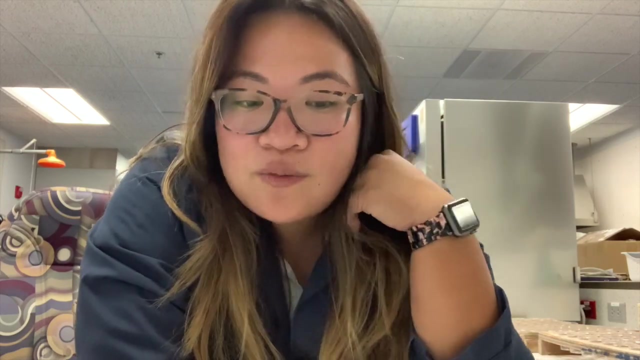 alerts. I basically do tests to lift those boiled water alerts so that you guys don't get sick when you drink it. Another big part that I do is effluent testing, which is toxicology, So wastewater plants when they treat their water, they discharge it into a body of water. 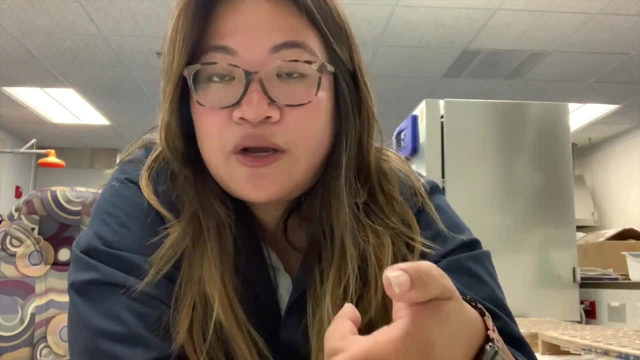 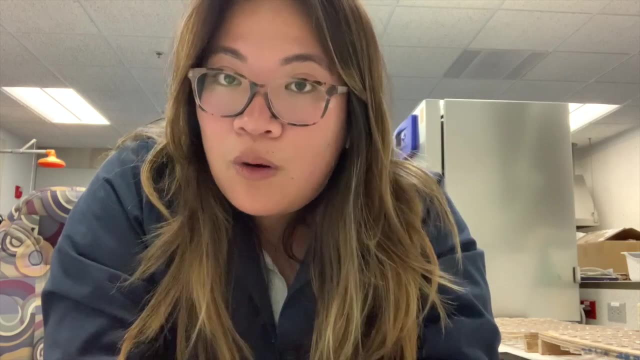 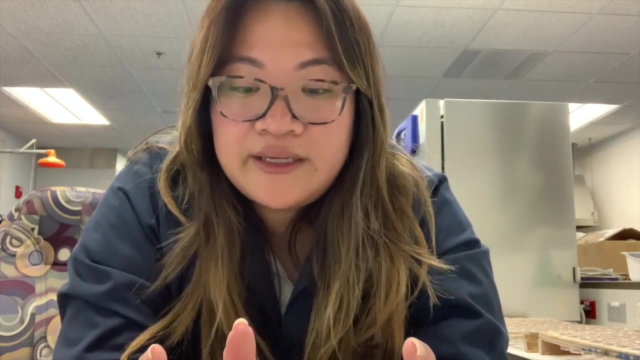 In my city we discharge it either into the ocean or a river or an area where they both mix. but we make sure that that water that's getting discharged is safe for the ecosystem. So we test it on small organisms: It's cereals and promulas, which are water fleas, and fishes if they're. 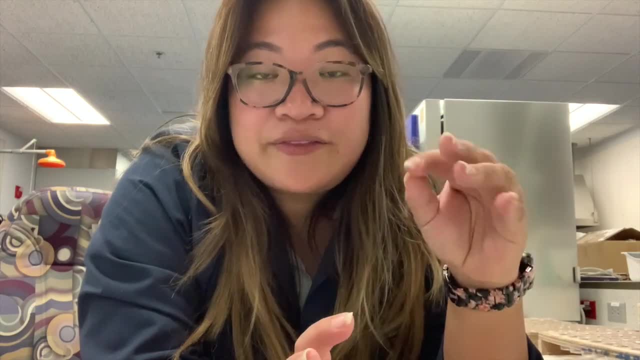 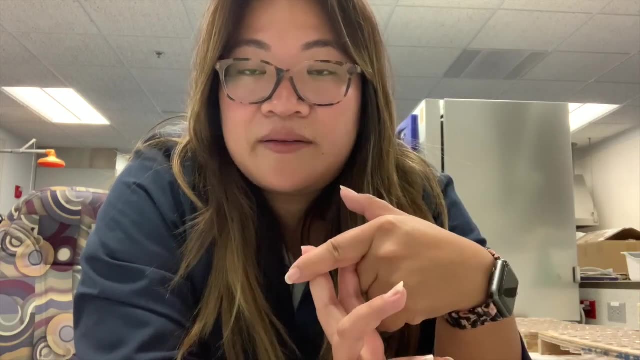 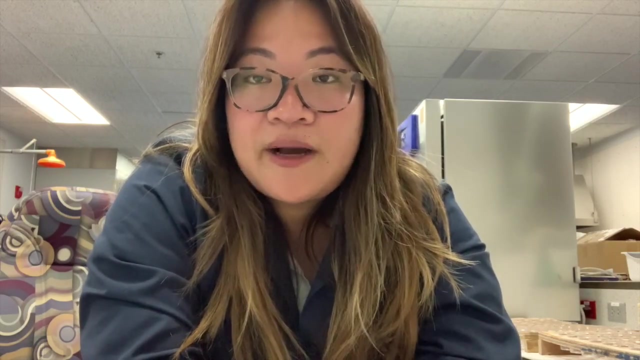 discharged into fresh water. If they're saltwater, it's brine or it's mysids, which is small, small shrimp and beryllinas, which are also small fishes. So we test on those because if they're affected by the effluent and they die, the bigger fishes that feed on them will also die. 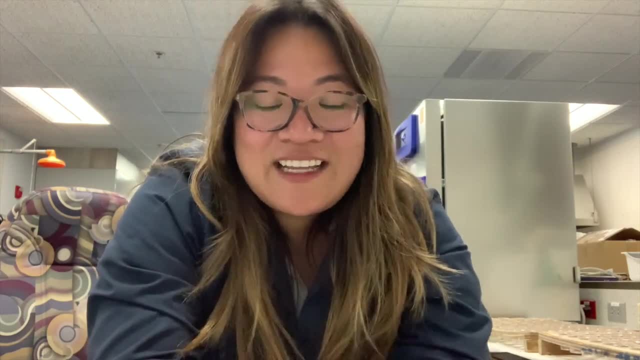 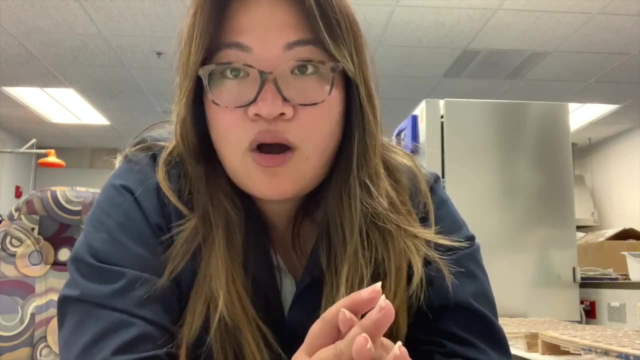 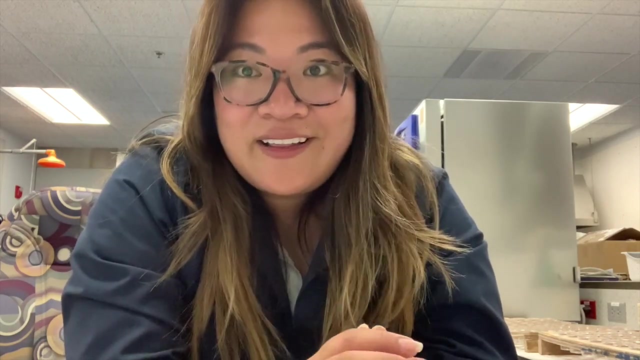 and so that will totally kill the environment, And so we want to make sure that doesn't happen. Another big thing that we do is microbiology testing on the effluent as well, just to make sure that the bacteria doesn't totally kill the ecosystem either and to make sure that people that 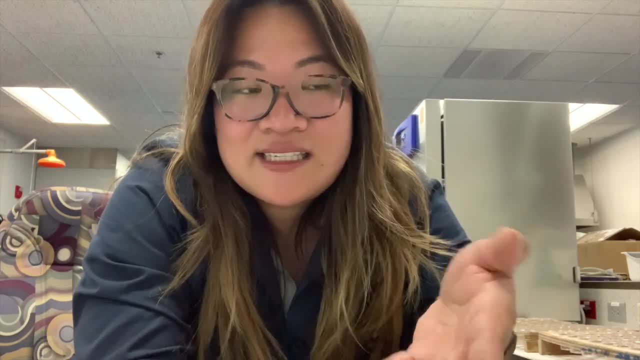 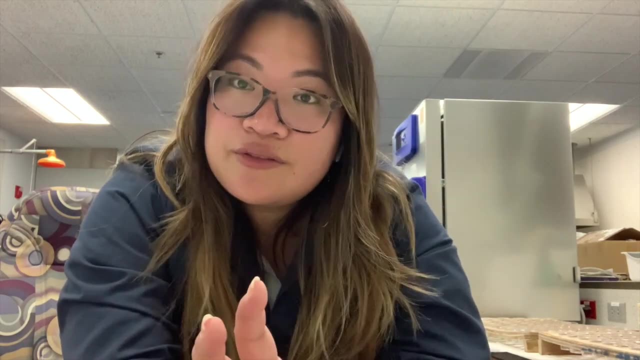 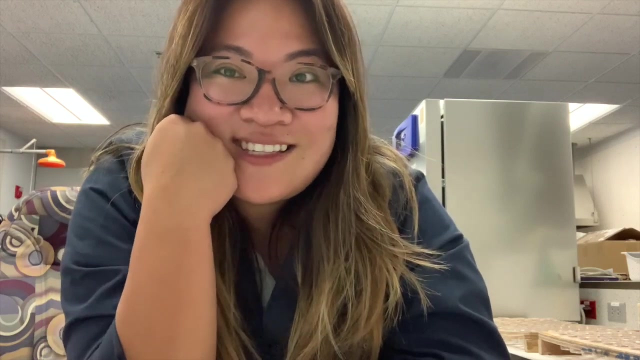 are that decide to swim in it. they don't get sick and we also do micro on reused water, So it's water that basically waters the получится horses. here in Florida we want to make sure that's safe and you know we have kids that run. 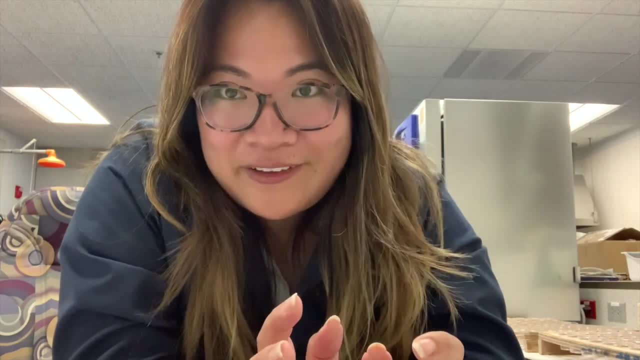 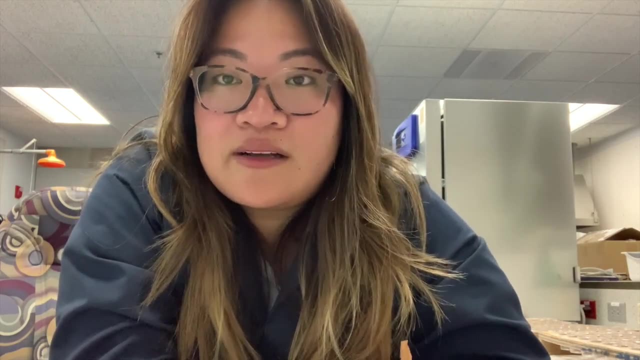 through sprinklers during the summertime, so we want to make sure that water is clean, um. but I figured that today was a great day to bring you guys with me, because I'm kind of alone in my department today and I don't know my manager isn't here, so I figured I'd have something a little bit. 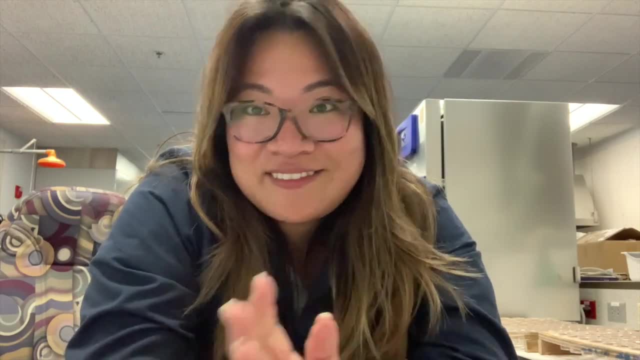 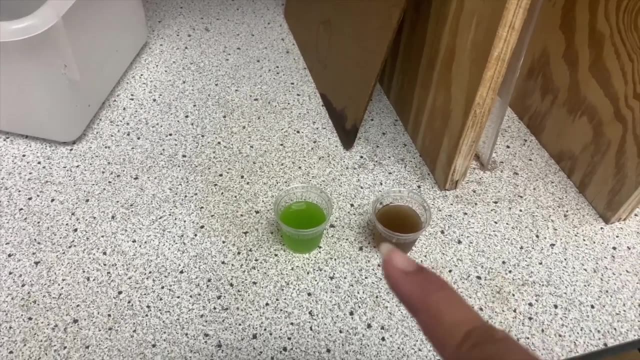 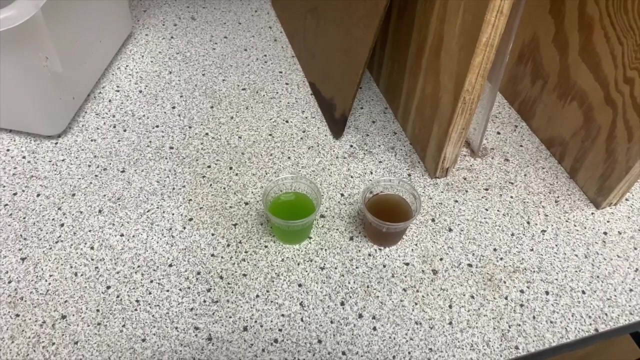 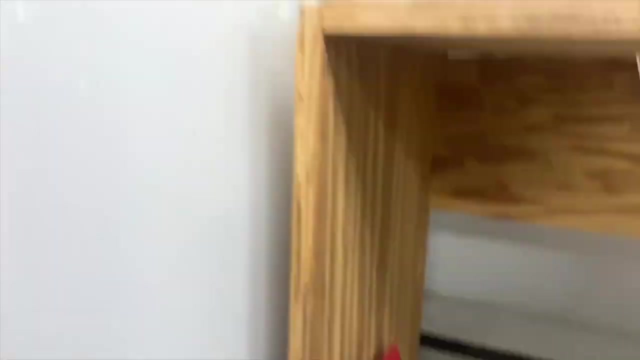 different with you guys, so come with me. so first thing. first is that I am feeding our cereals- the one on the left is algae and the one on the right is ytc- and I'm basically going to pipette the um food to a beaker full of cereals. it's full of moms and their babies, but we have this on hand. 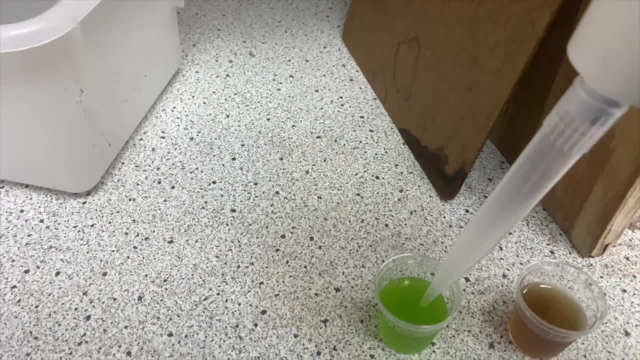 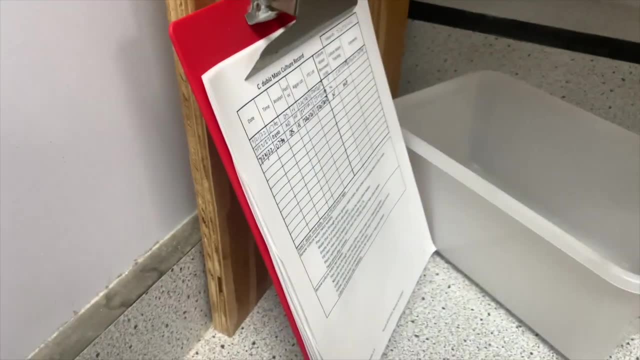 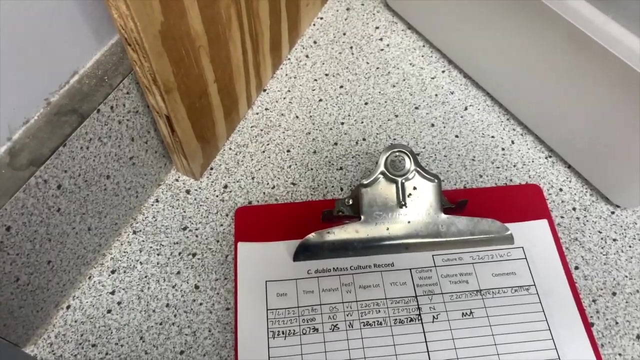 just in case we need to start a brood of cereals and we like having a brood of cereals cultured for two weeks prior to actually using them in fresh water tests. so that's why we have this for quite a while. so I'm just filling out a few things. 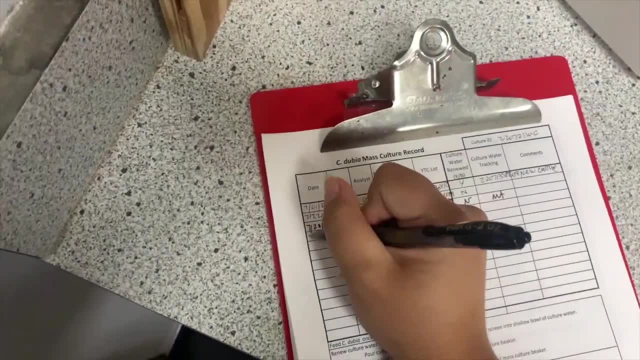 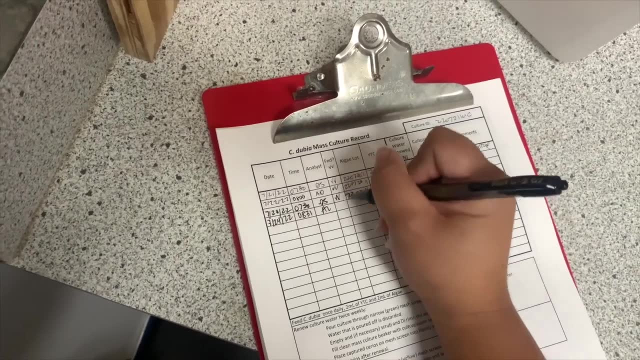 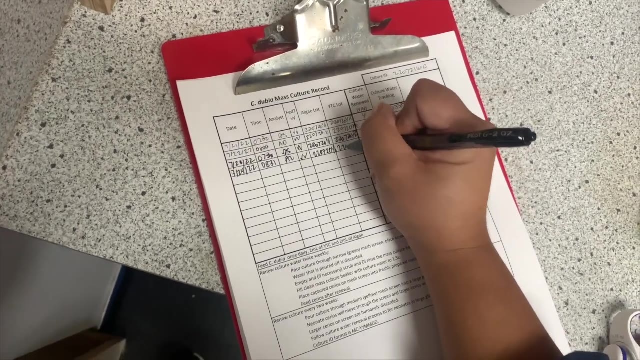 on this clipboard, basically the date, time and the tracking numbers for the foods that we use. we record everything in the lab. we just want to make sure we see why a cover our butts. we just want to make sure we can trace everything that we use for these organisms. 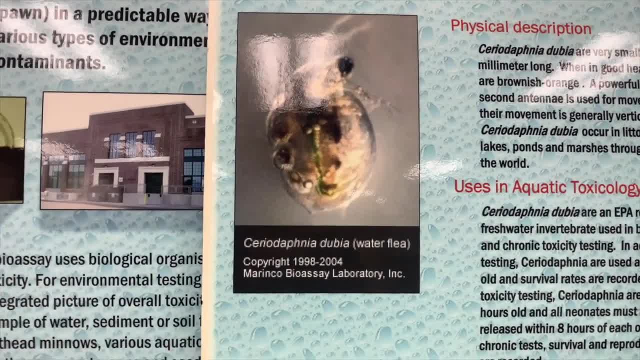 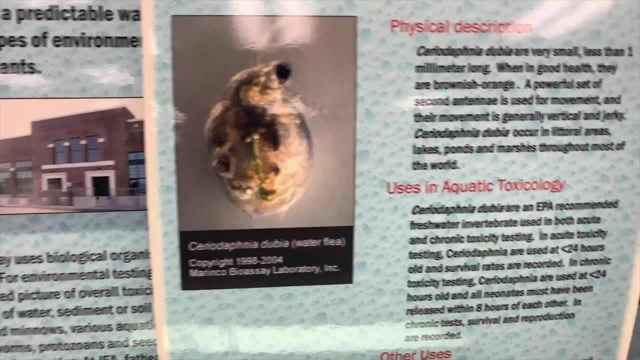 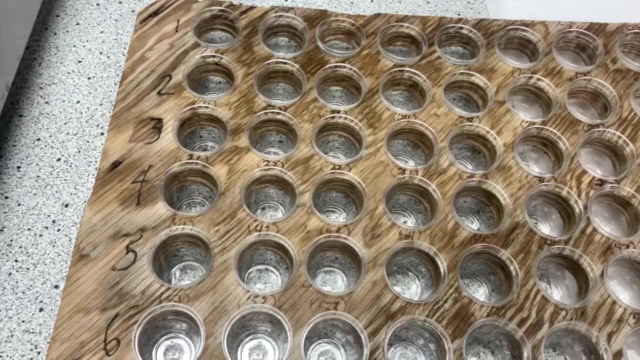 so here's just a magnified picture of the cereals. they literally look like that. they're clear and brown. and then right over here to the side is the freshwater fish that we use, the promelas, and so that's kind of a magnified picture as well. 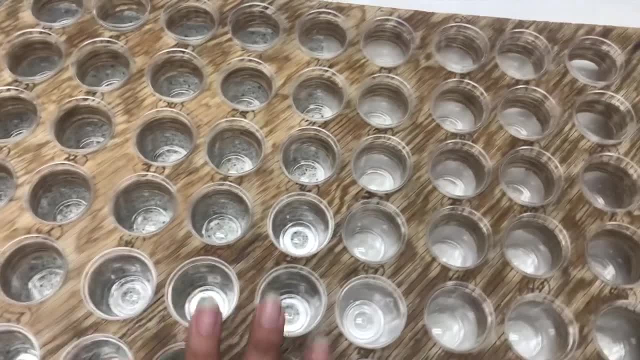 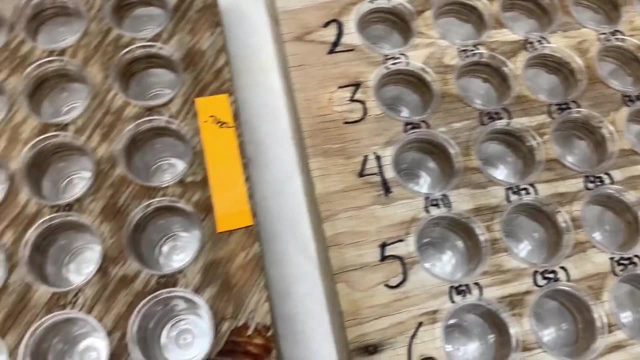 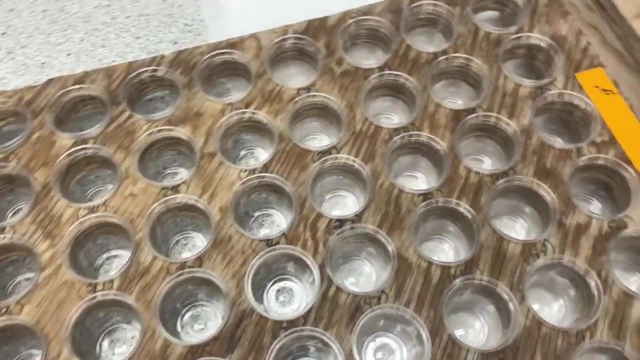 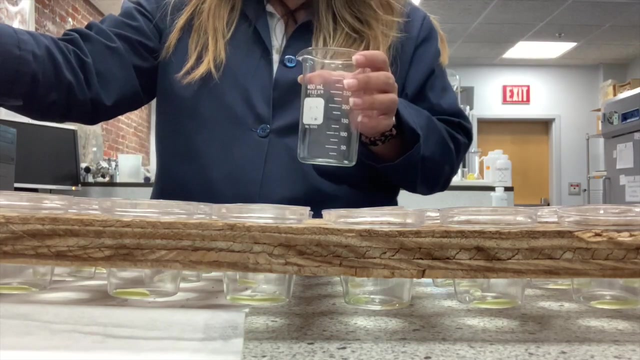 so this is a brood board. um, each cup will have one mom and each mom will basically have babies for a course of two weeks. every day we count how many babies they have and then we transfer them into new brood boards. you can kind of see that there's algae and ytc in each of the cups. so next I'm going to put the 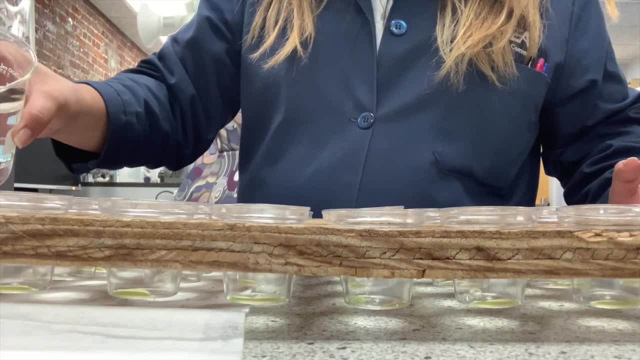 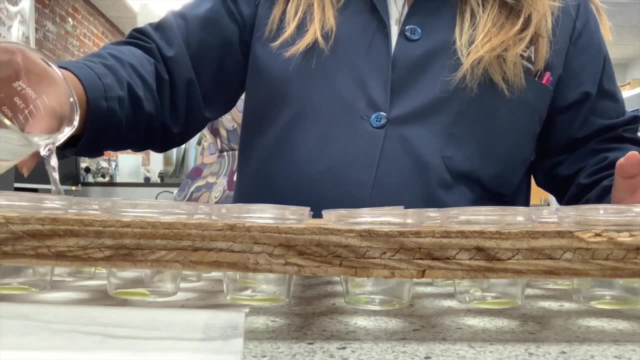 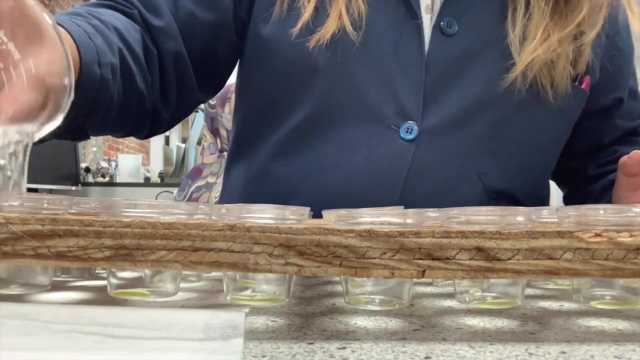 fresh water that we make in the lab into the cups um. so each brood board has 60 cups. so in total every day we count 120 cereals and count how many babies they have. typically on the first through the third day they don't have any babies, but then on the fourth day, that's. 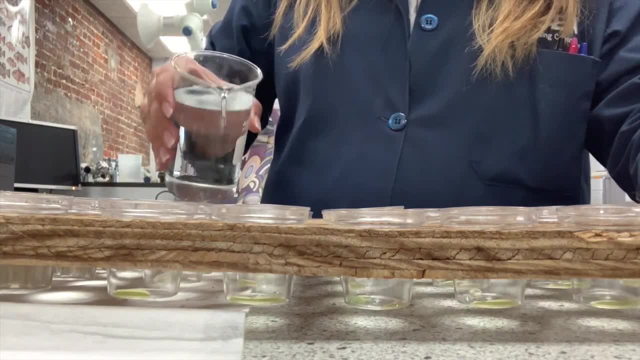 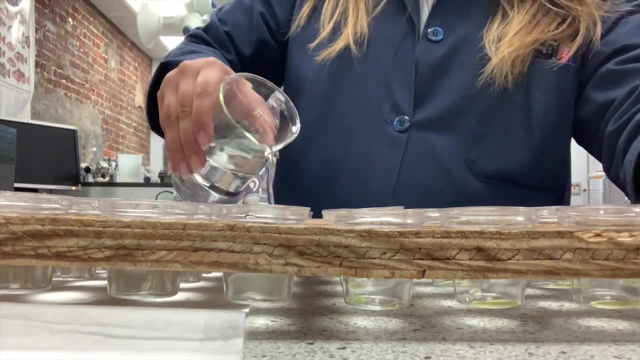 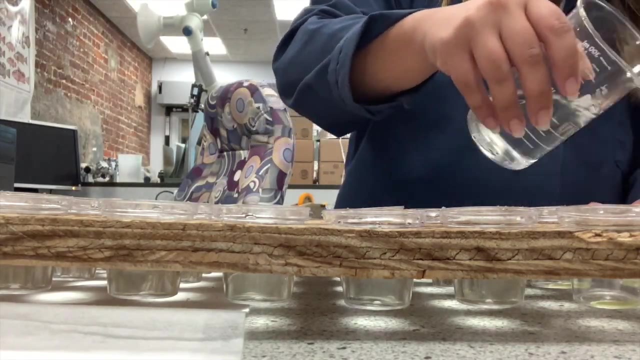 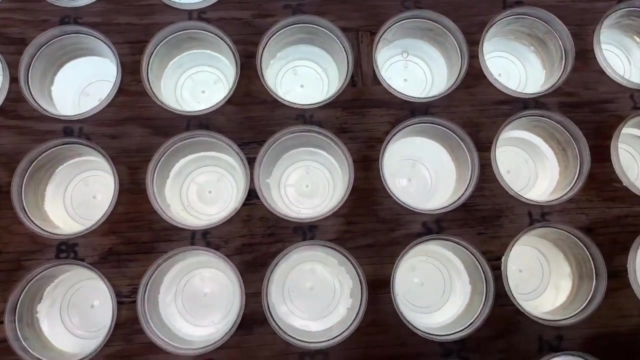 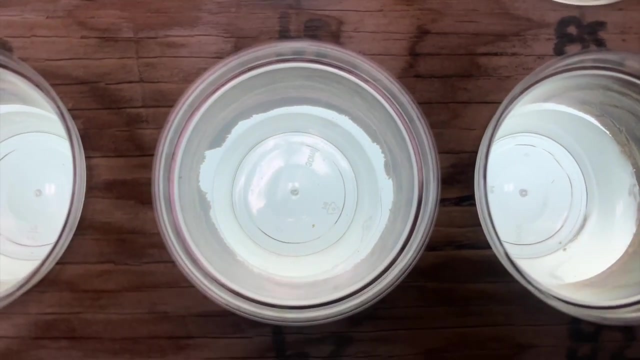 when they really pop off and they start making babies. I've seen them make about like 20 babies one time, so they're pretty healthy. all right, ladies and gentlemen, get ready to pull out your magnifying glasses, because let me know if you guys can spot the cereal. it is a tiny little dot, kind of um, swimming around in. 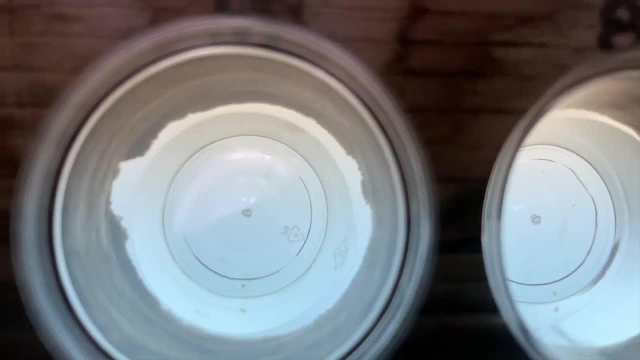 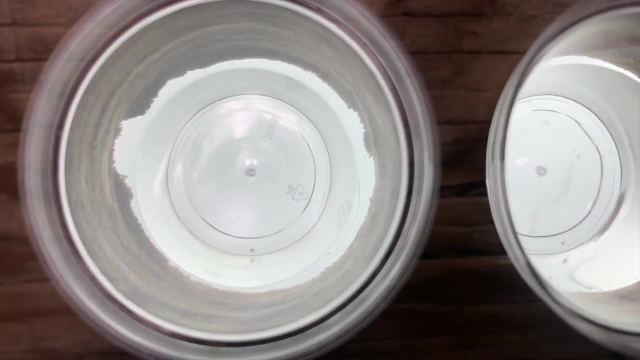 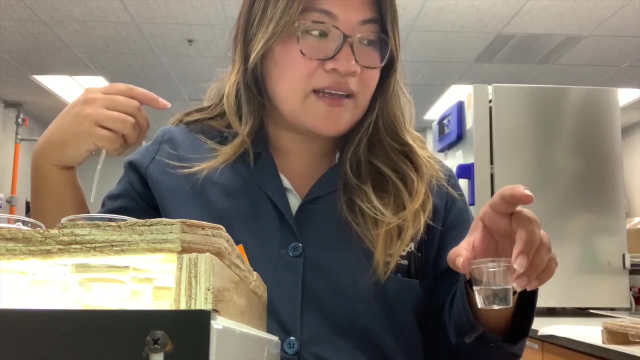 it's like in a really jerky motion. so thumbs up if you see it and comment down below. if you do so, we count the amount of babies that they have, which are even smaller dots. okay, don't mind me, I was trying to explain and record at the same time. 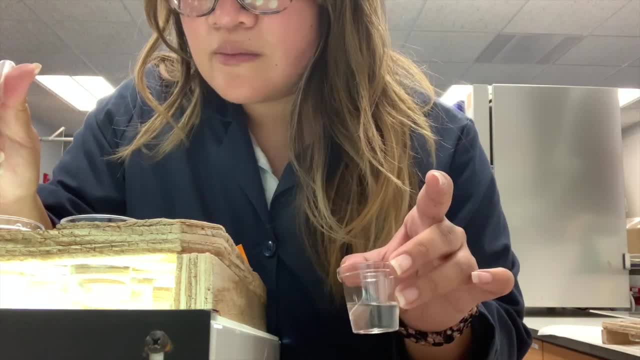 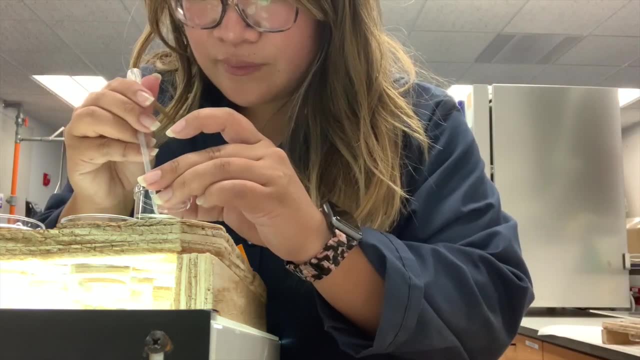 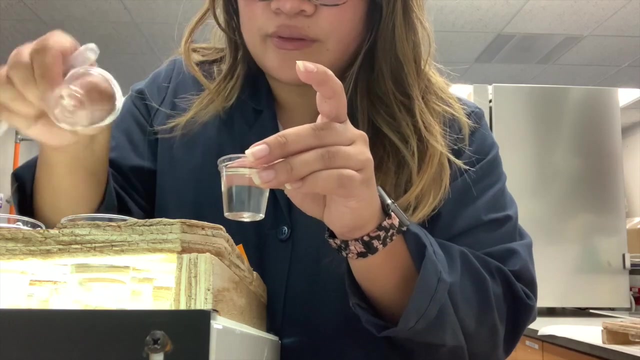 but that incubator behind me was just way too loud and it didn't sound that great. but after counting the cereal babies, we're going to transfer the mom into a fresh board. that's the one where I added the food and fresh water in. so what I do is I take the cup from 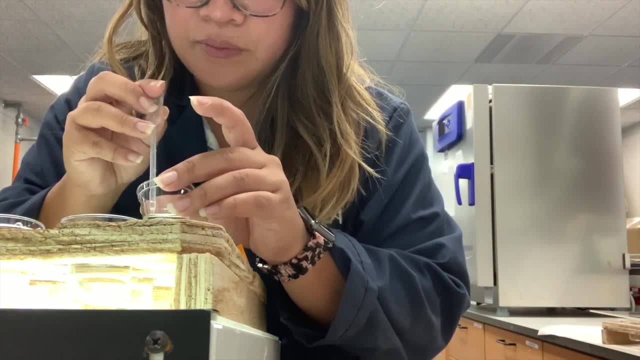 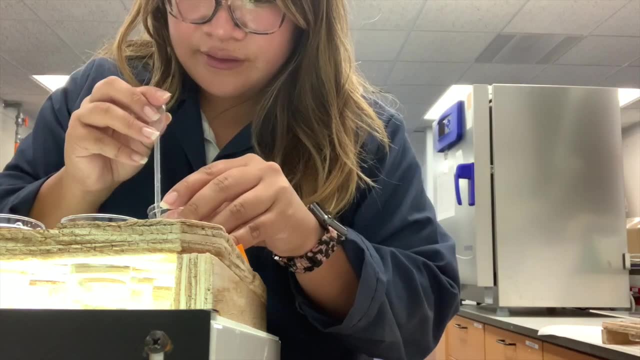 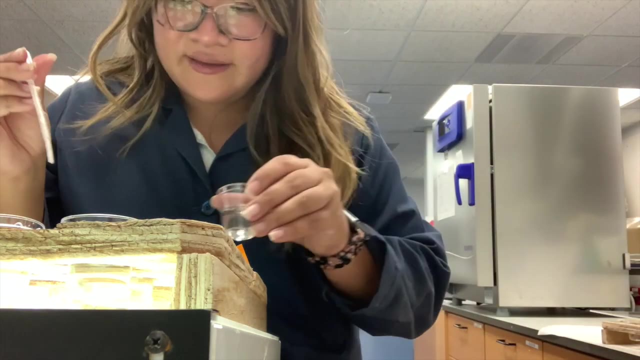 the old board, bring it up to the light board, like what I'm doing right there, and then transferring the mom into the new board. we use transfer pipettes and we have to be really gentle because these cereals are so sensitive and we could kill them at any moment. we can't even wear perfume or wear. 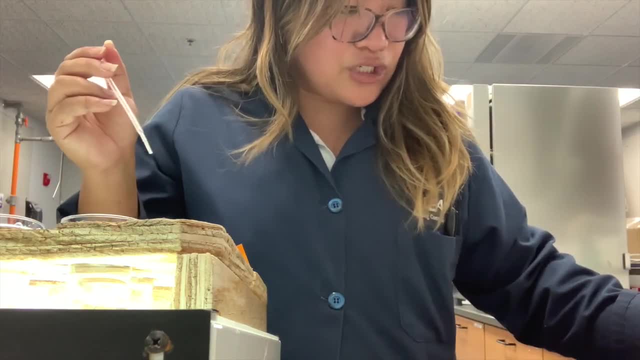 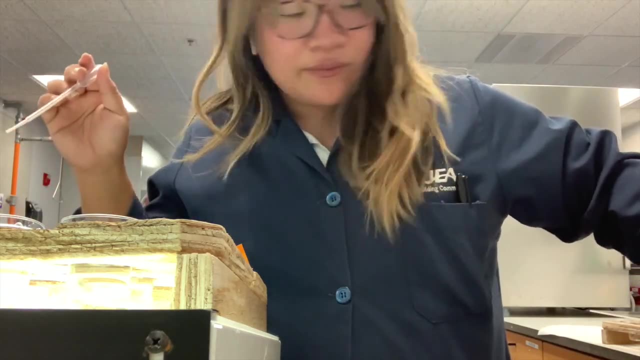 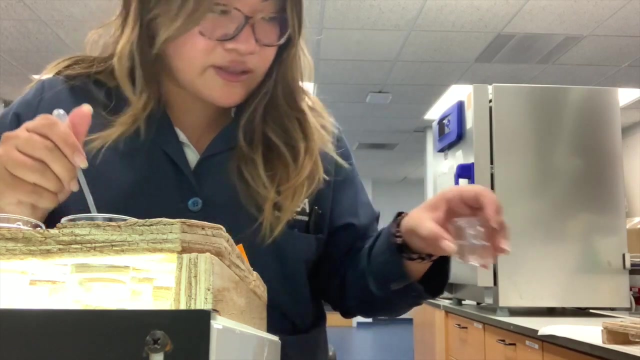 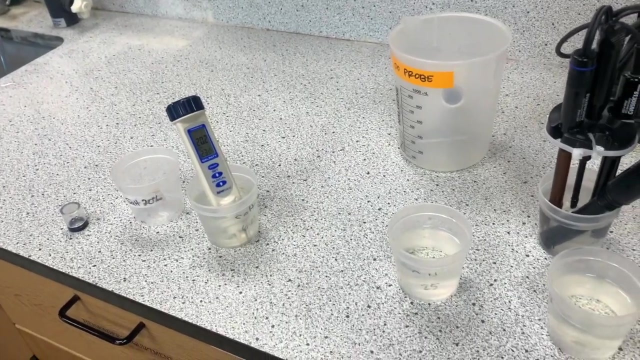 scented lotion to the bio lab because they're that sensitive. we've had issues for like six months and then finally we realized that we couldn't even wear gloves or perfume or anything. so we're all dirty lab rats in the biology department. so for today, we have one bioassay. 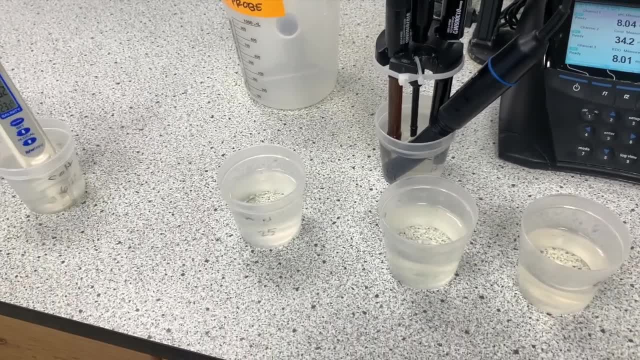 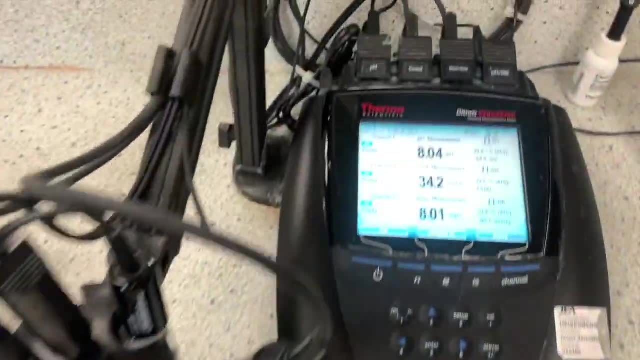 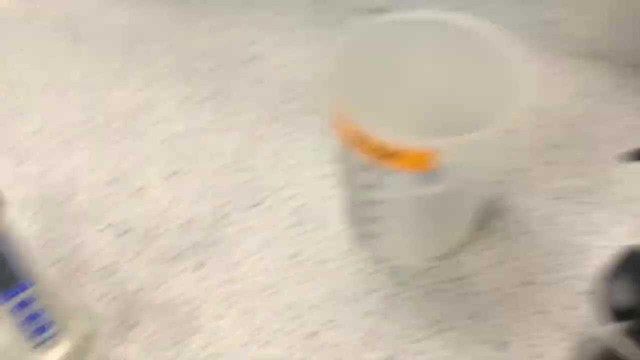 test for one of the wastewater plants that discharges into the atlantic ocean. right now I am doing the pre-exposures and basically we use this meter right here, heisenberg, to make sure that the dissolved oxygen do and the ph are within the acceptance criteria, and we also check the 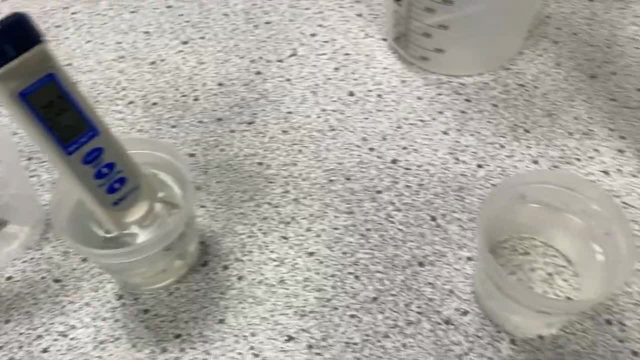 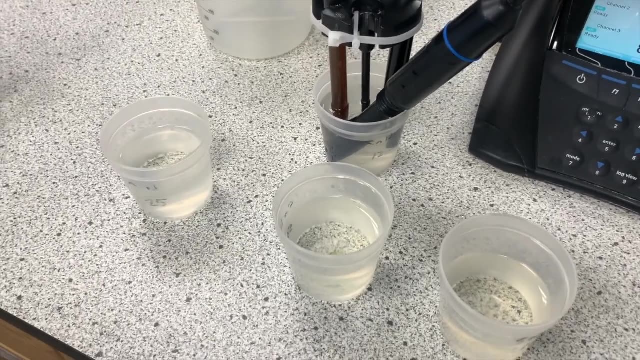 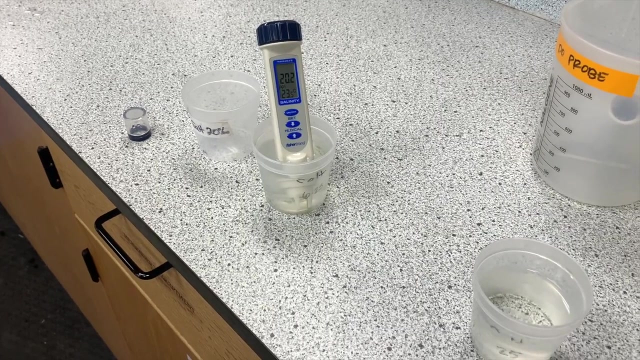 salinity of each dilution. so we have six dilutions um. one is a control and every experiment has to have control, which is the baseline, and then a 6.25, 12.5, 25, 50 and finally the 100 percent dilution. we just want to make sure that. 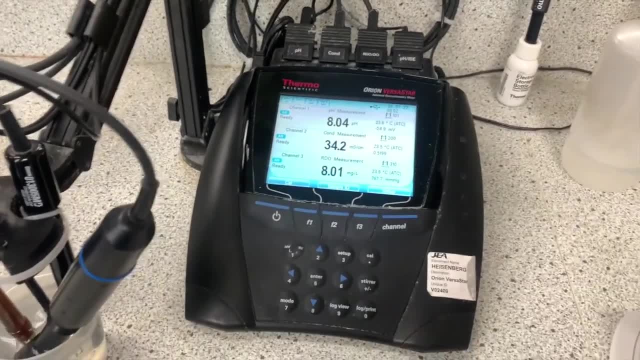 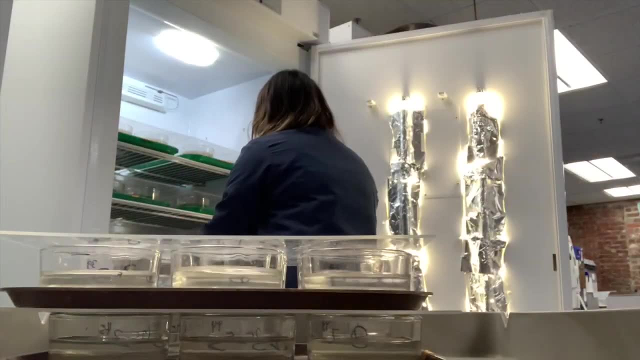 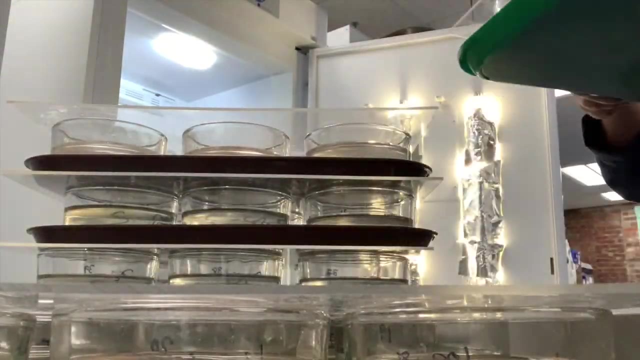 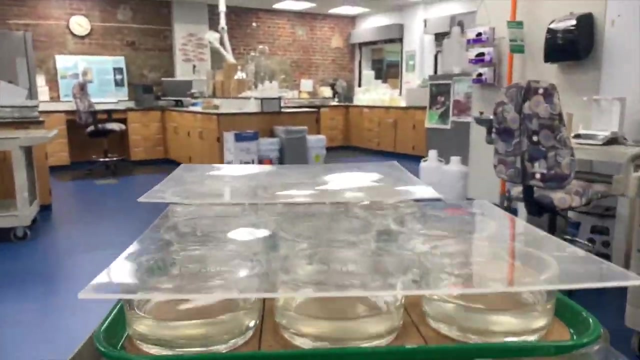 at every dilution. none of the organisms die and it's safe for us to discharge into the ecosystem. so the first organism that we are going to work with are the mysids, and the mysids are basically tiny little shrimps that we expose to the dilutions. um, each chamber is a little bit. 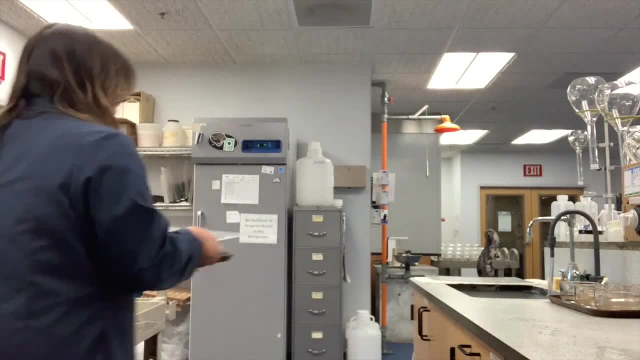 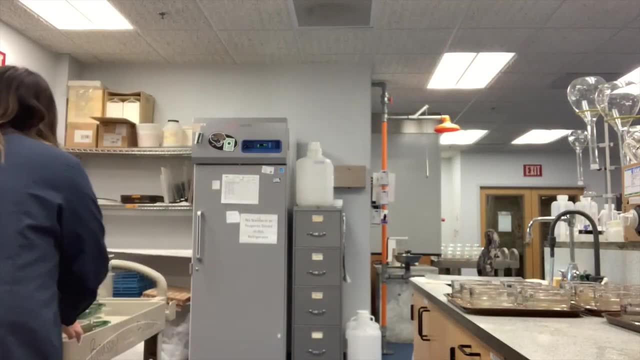 smaller and they're going to have a very small amount of heat that will be released, and then they're going to have a very small amount of oxygen and they're going to have a lot of oxygen in there. so that's why we're going to have a lot of oxygen in there. so we're going to 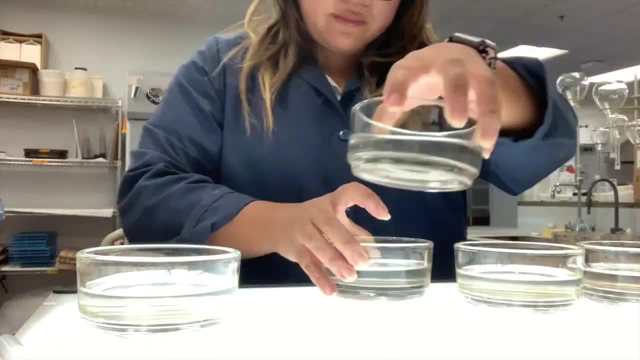 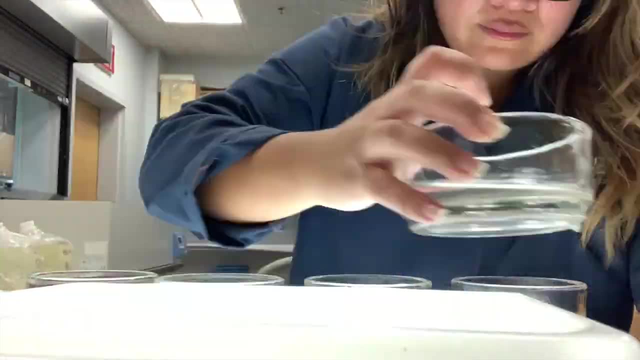 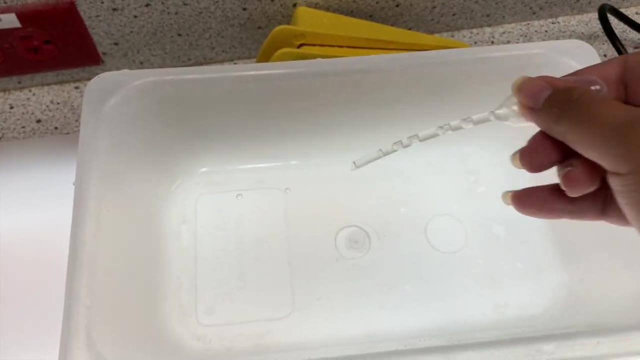 will have five mysids, and so we just keep track of how many stay alive and we pour off the water, as you can see here, and then we take their post exposures. we just want to make sure their values are good as well, and, as you can see, one of 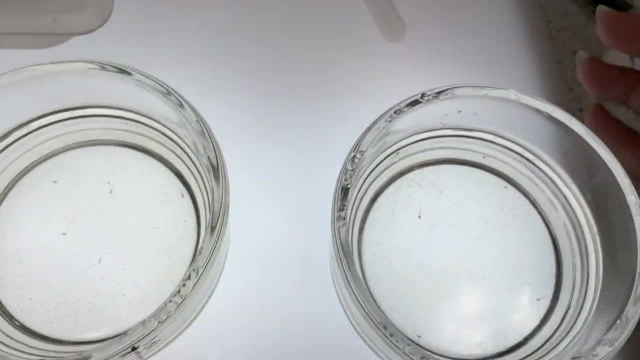 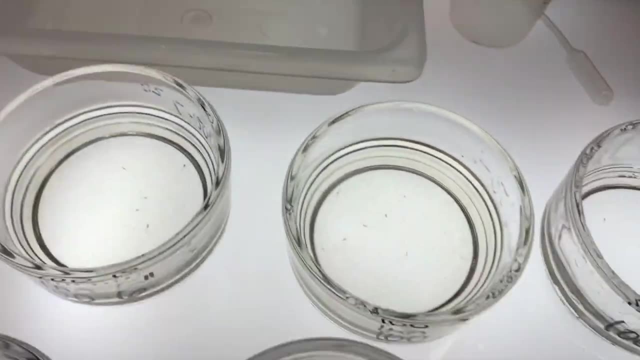 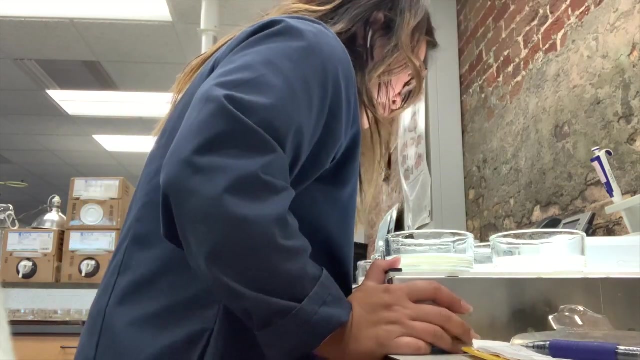 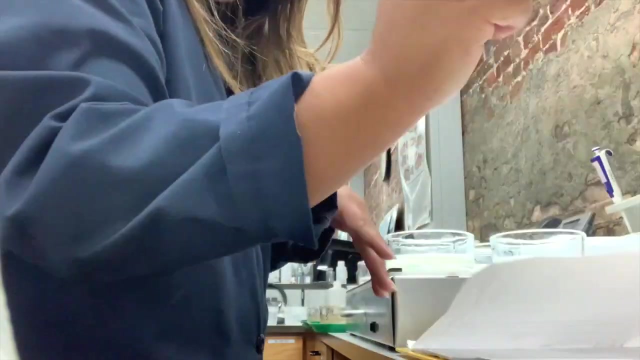 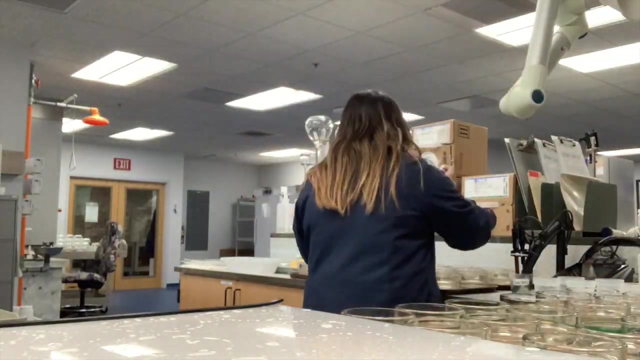 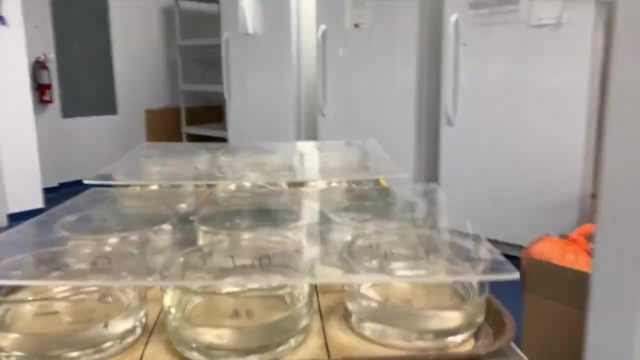 the mysids escaped the chambers and so I put one back you. so once I've renewed all the mysids, they are fed with brine shrimp and we're putting them back in the incubator, and then next we'll be pulling out the fish so that we can renew them. 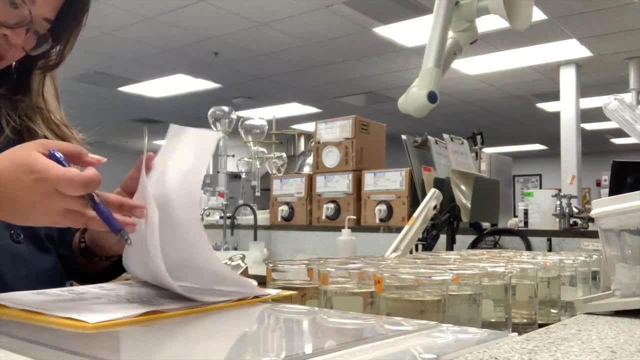 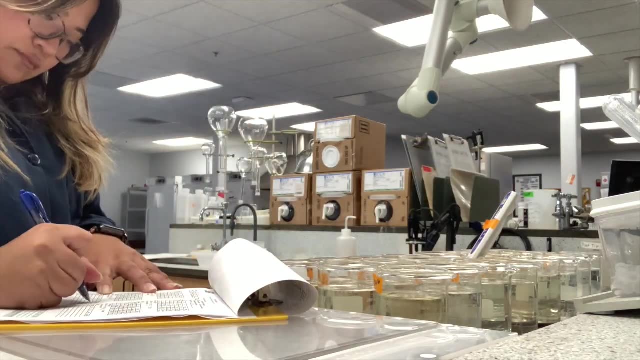 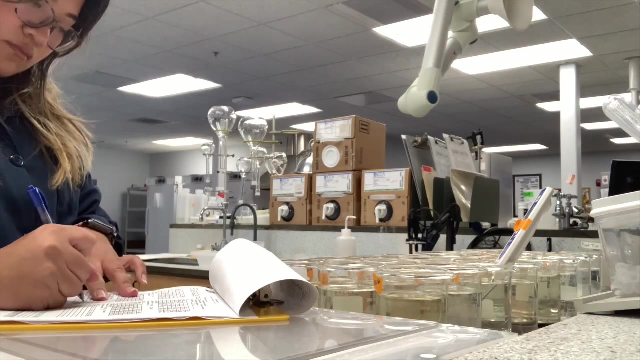 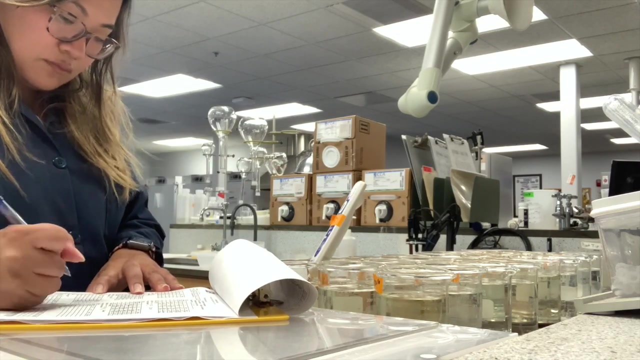 so, as you can tell, there's a lot less chambers for the fishes than there are for the mysids. the mysids had eight chambers and each one had five mysids, but for the fishes there's four replicates and 10 organisms in each chamber, and you'll see how crazy those guys are in the 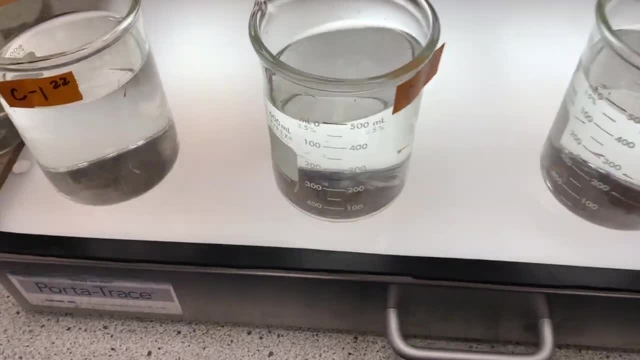 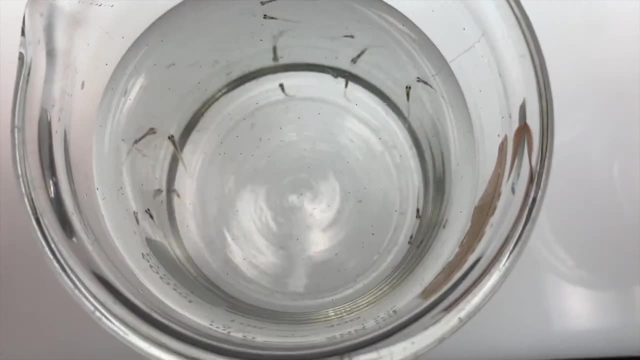 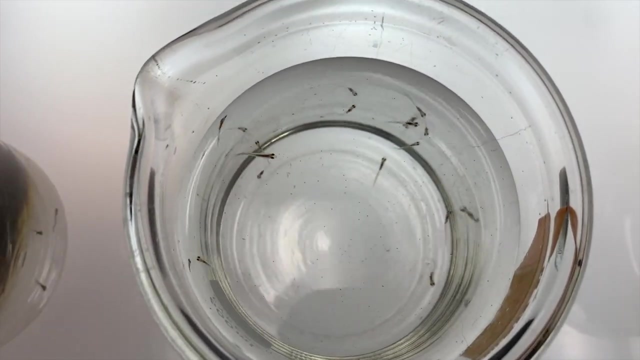 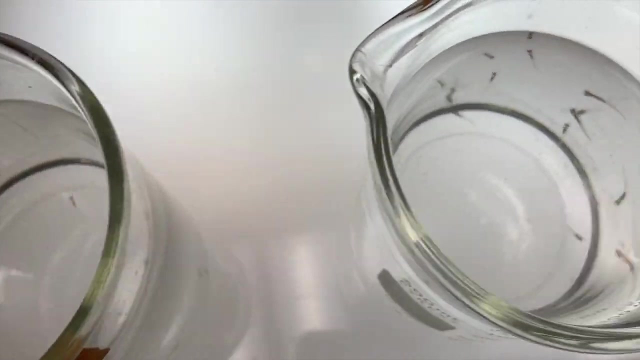 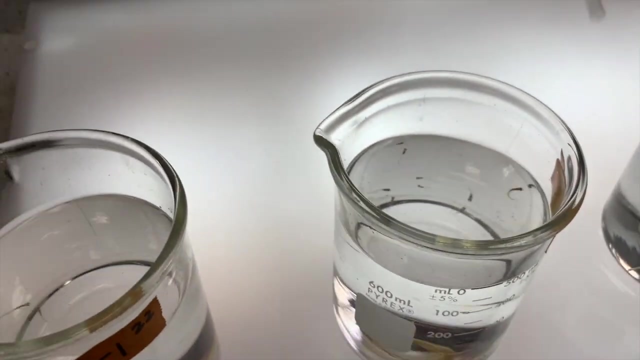 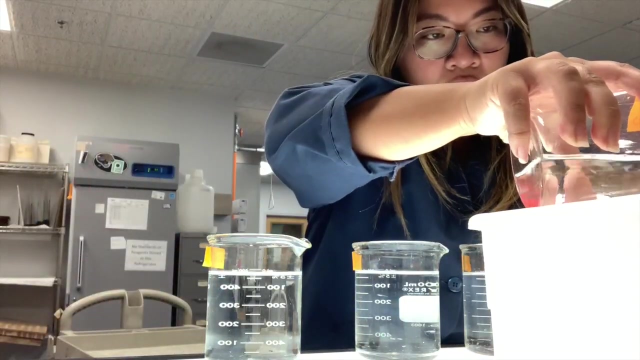 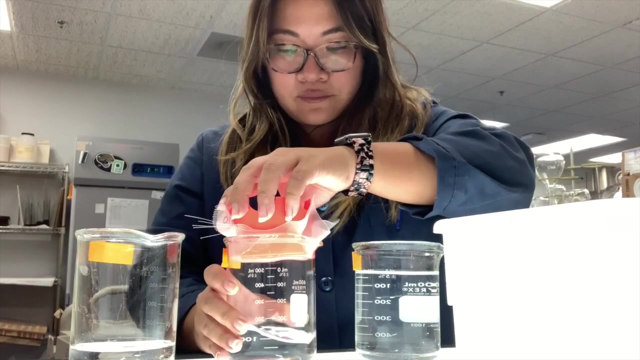 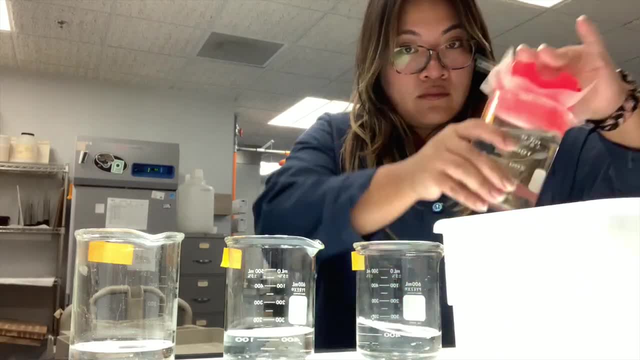 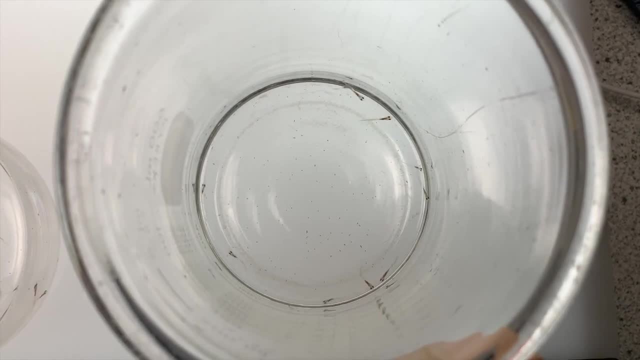 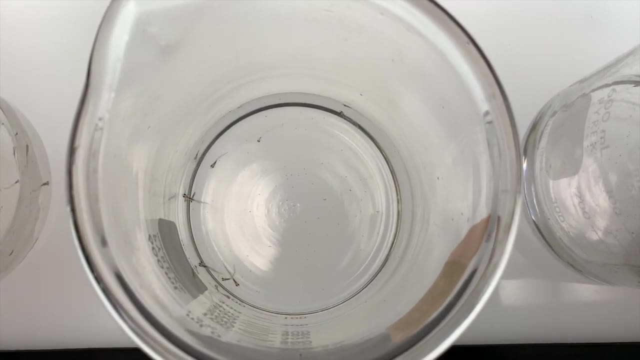 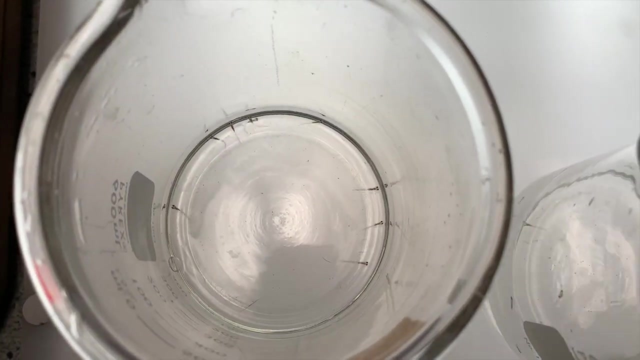 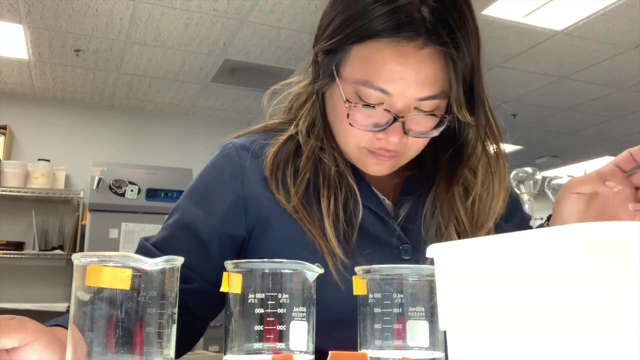 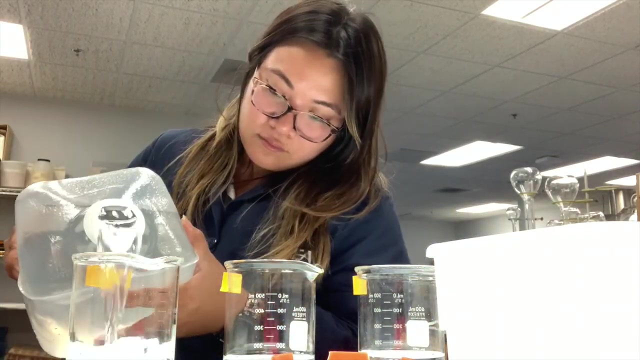 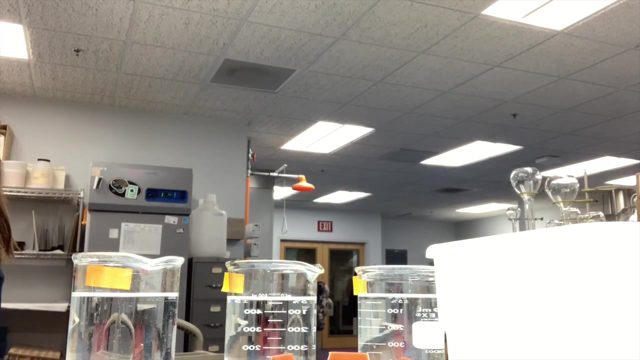 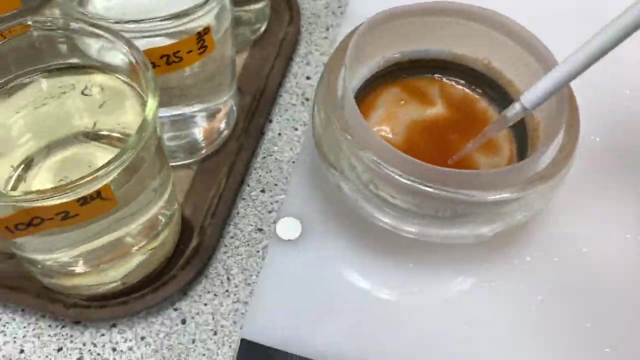 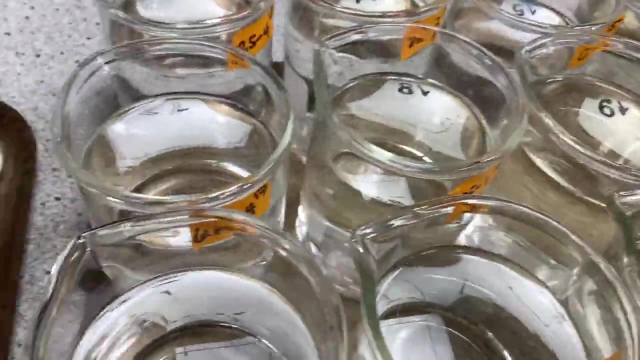 number of organisms in each chamber to make sure none have died, and then take the post exposures on the old water. So after the renewal process we feed the fishes as well, and then they also go back to bed, and then we'll see them again the next day and start the whole process again. 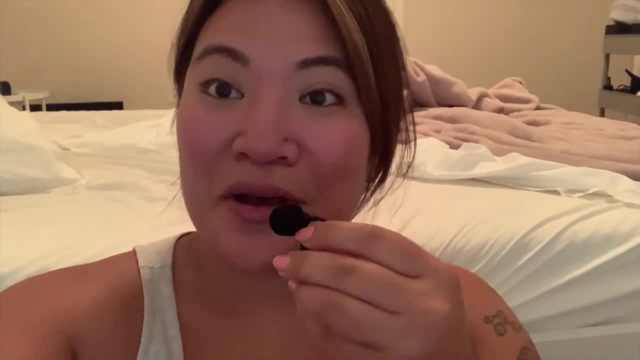 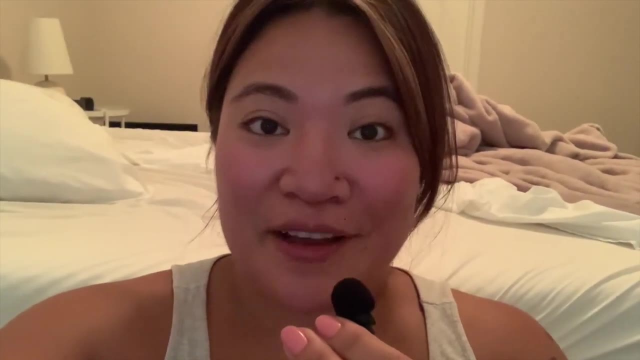 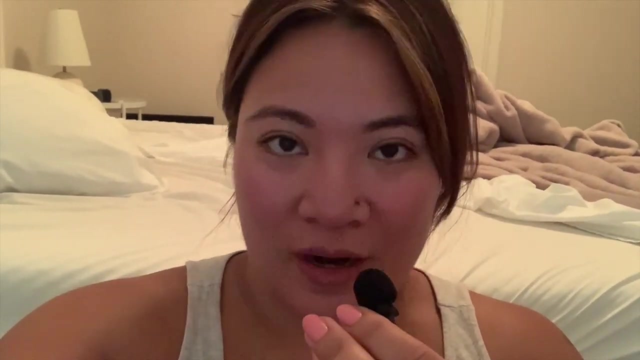 Hi, hello. this is post-filming and post-editing, Isla. I just wanted to say thanks everyone for tuning in. I split this video up into two parts: one for the bioassay, which you guys just watched, and another for the microbiology. 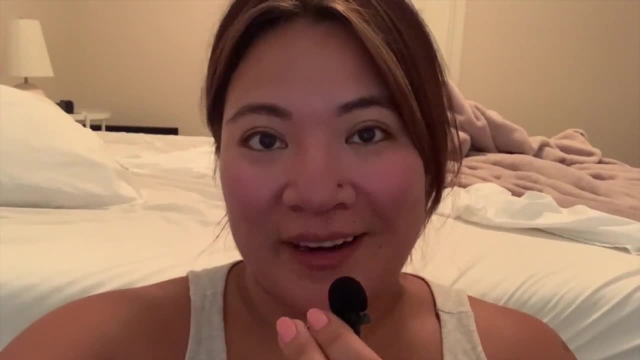 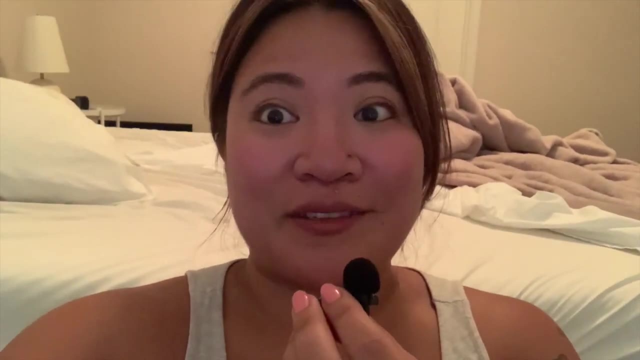 I wasn't entirely too sure how this video was going to work out or how you guys are going to react to it, so I'm not going to post the microbiology part Until you guys want to see it. this was really fun to make. 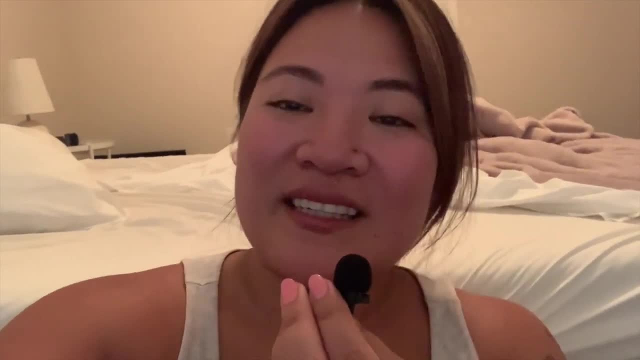 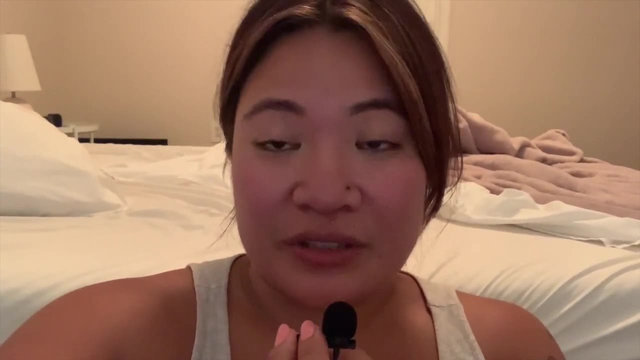 It was really weird to ignore the camera and work at the same time, but I just wanted to share this part of my life with you guys and share what I wanted to do, because I think it's really cool and it's really important. Water is so important.